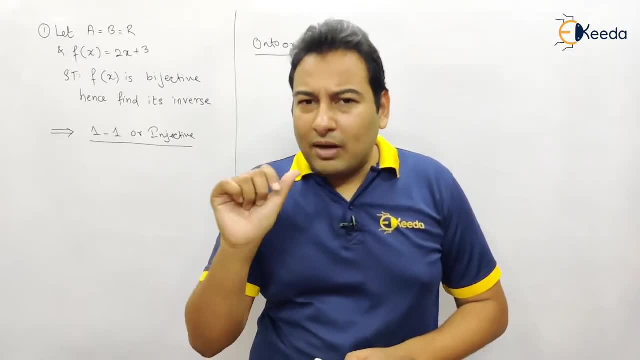 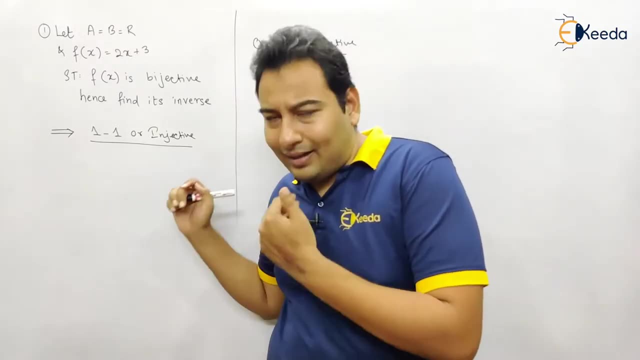 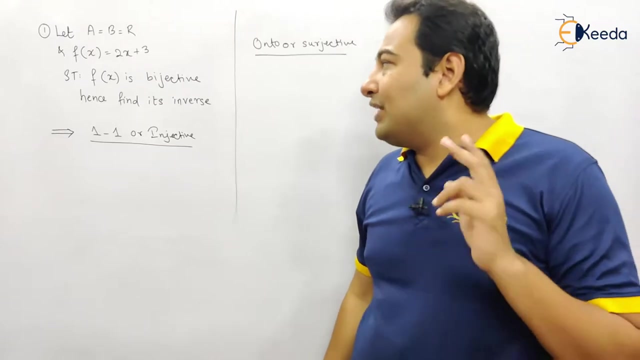 First of all, you need to remember a point: If a function is bijective, then only you can find its inverse. So we'll prove it is bijective, then we'll find its inverse. So let us start For proving that the function is bijective. two things we need to prove that the function is: 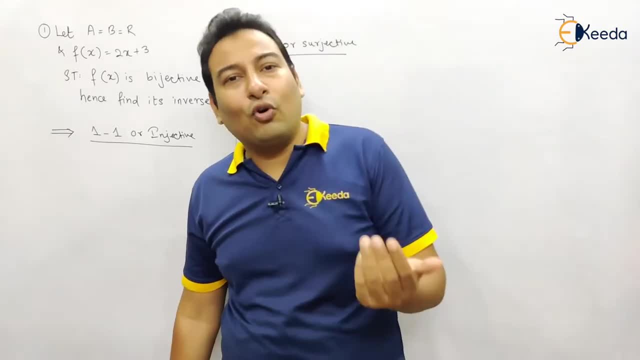 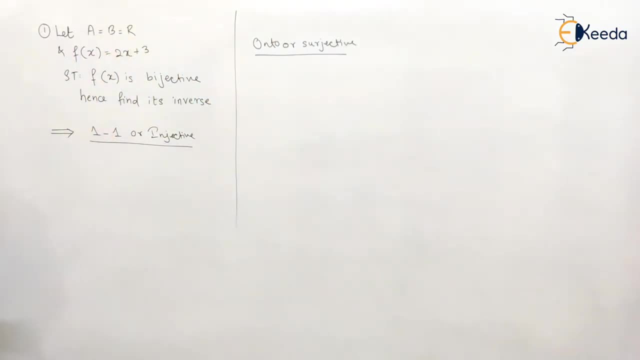 one-to-one and function is onto. Because if the function is one-to-one and onto both, we can conclude the function is bijective and its inverse exists. So let us start with the one-to-one. one-to-one procedure. what is the definition of one-to-one or injective? the definition says: 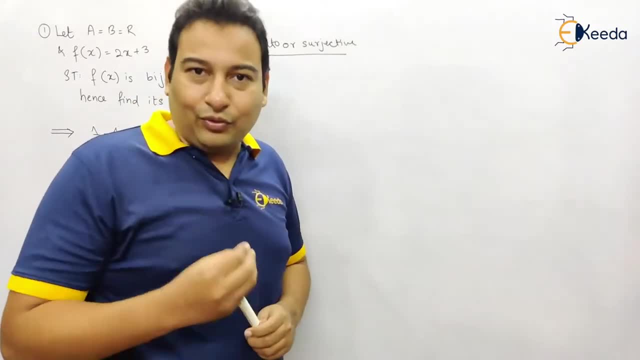 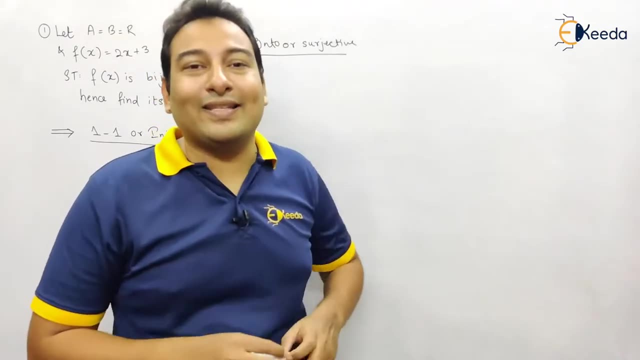 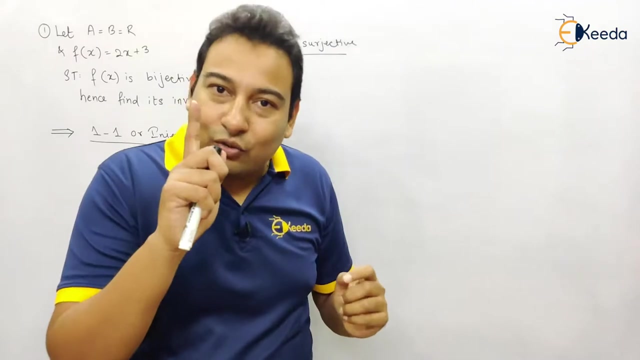 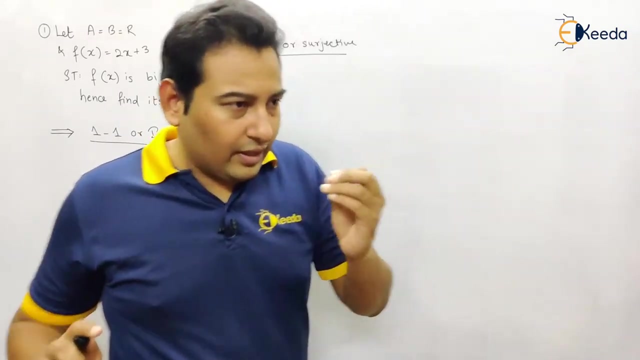 different elements should have different image, or this is what we have learned till now: different elements should have different image. or you can say: if the elements are same, their image is same. that means if there is only one element, or, in short, you can simply say, one element will have one image, that's it. so let us start first of all. 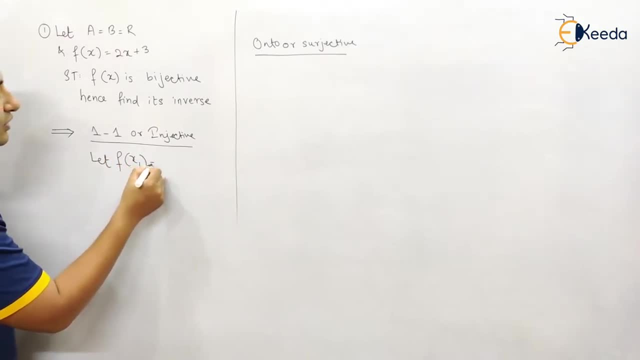 what we'll do. the procedure is fixed. we'll always start with this statement. it is always fixed in all the problems and we will prove this. therefore, we'll conclude: function is one-to-one. so what we did? we assume that there are two different elements, x1 and x2, and their images same. 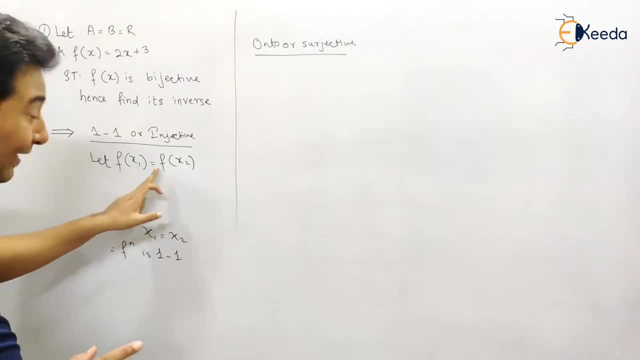 x1 and x2. both are different elements but they are the same. so we assume that there are two different elements, x1 and x2, and their images same. x1 and x2: both are different elements but they are the same. so we assume that there are two different elements, x1 and x2, and their images same. 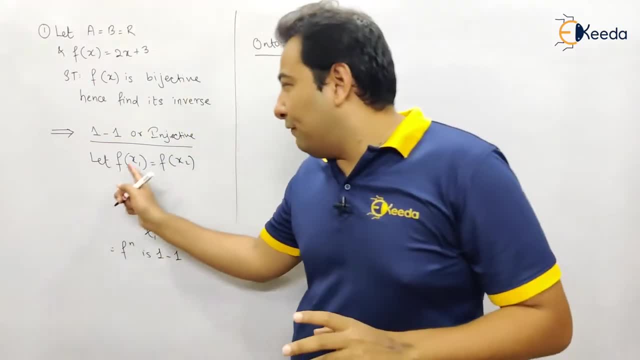 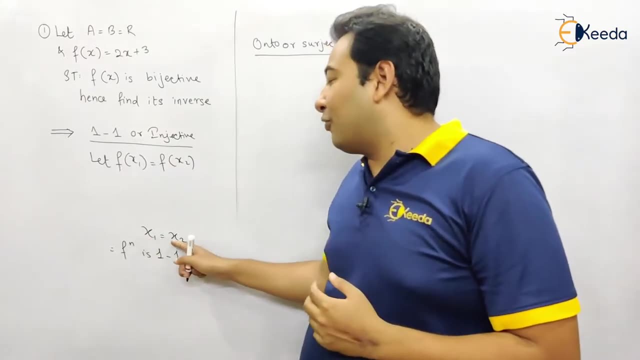 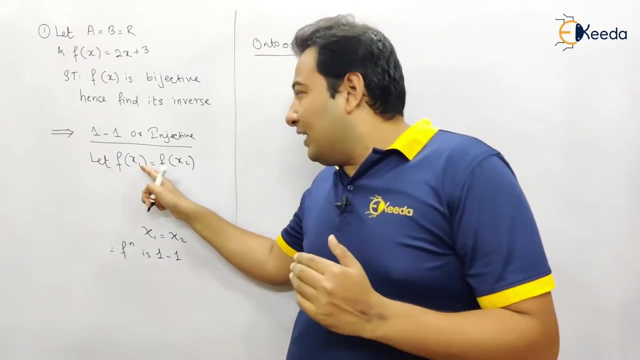 their images are same, which is not possible. if the elements are different, their image should be different. so, after doing few steps, what will conclude is: the elements are also same. so what? the? what is the statement saying what we're doing? we are starting with? there are two. 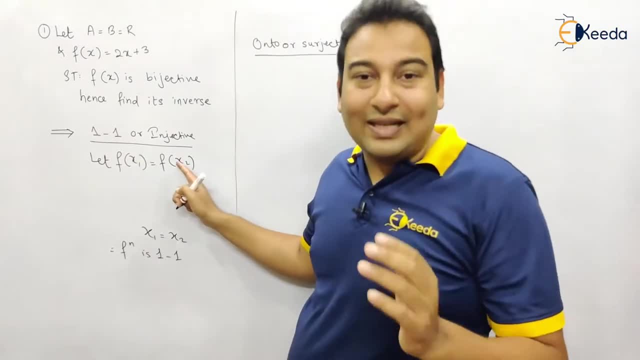 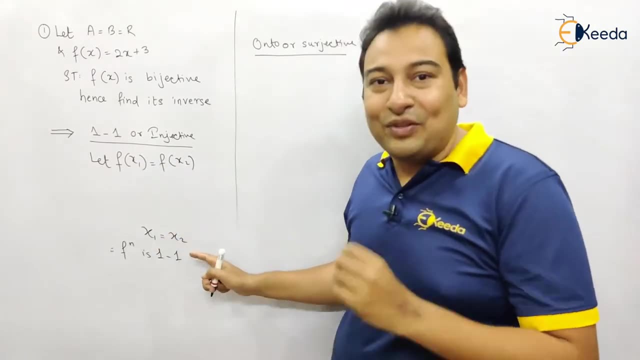 different elements with the same image, which is not possible, because if the elements are different, their image should be different and will conclude that the elements are not different. the elements are same. so that will indicate: if there is only one element- x1, x2- both are same. if there is only 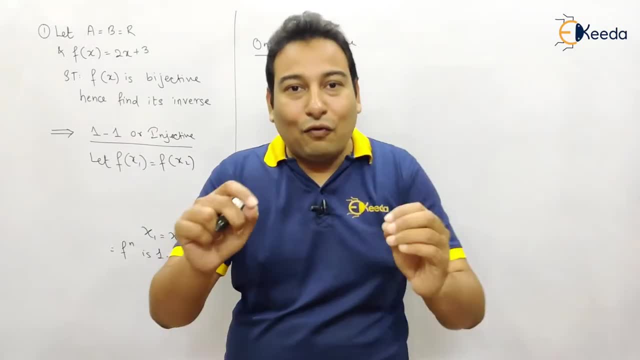 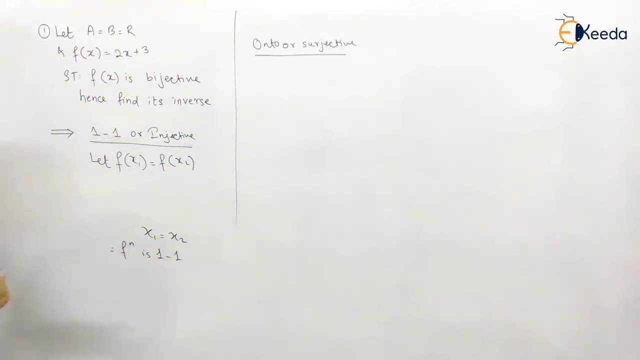 one element. there is only one image. so this is the procedure. if you understood the logic, what i said, well and good. if not, remember the procedure, we always going to do the same. let us start. so what you're going to do once, we're going to replace this x with x1, so this will become 2x1 plus 3. 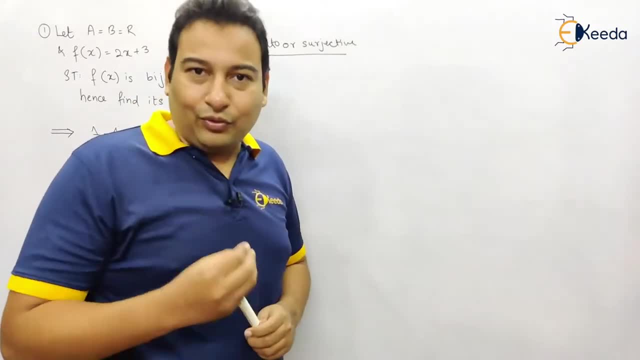 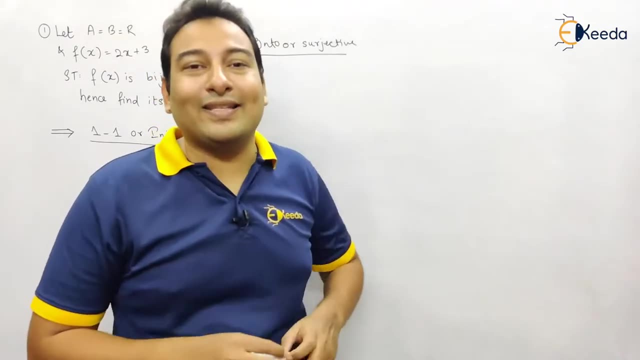 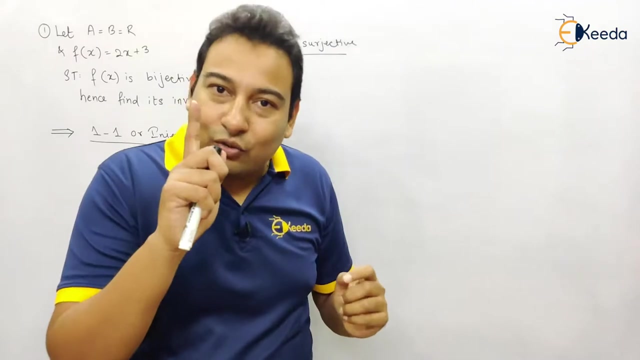 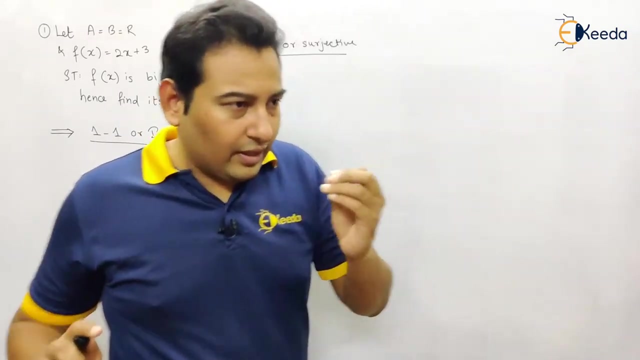 different elements should have different image, or this is what we have learned till now: different elements should have different image. or you can say: if the elements are same, their image is same. that means, if there is only one element, or in you can simply say, one element will have one image, that's it. so let us start first of all. 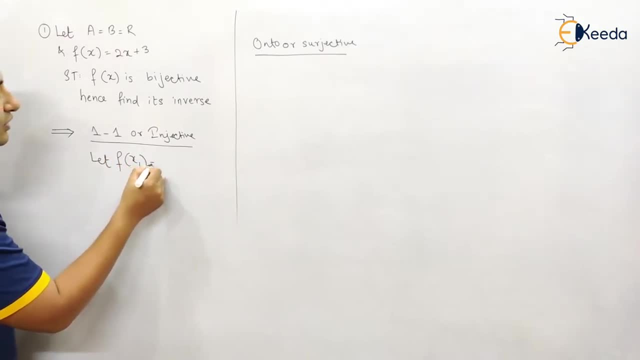 what we'll do. the procedure is fixed. we'll always start with this statement. it is always fixed in all the problems and we will prove this. therefore, we'll conclude: function is one-to-one. so what we did? we assume that there are two different elements, x1 and x2, and their images same. 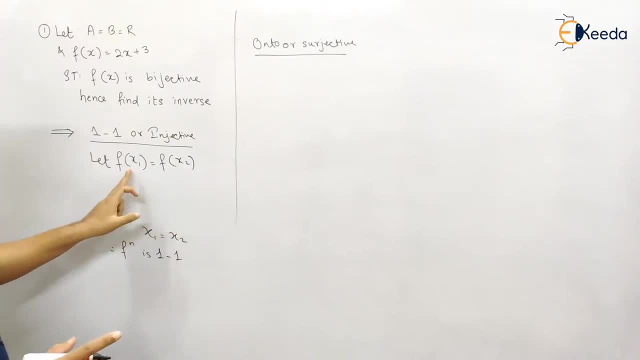 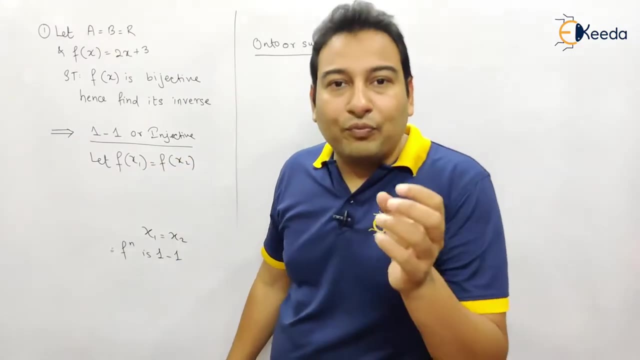 x1 and x2. both are different elements, but their images are same, which is not possible. If the elements are different, their image should be different. After doing few steps, what will conclude is: the elements are also same. What is the statement saying? 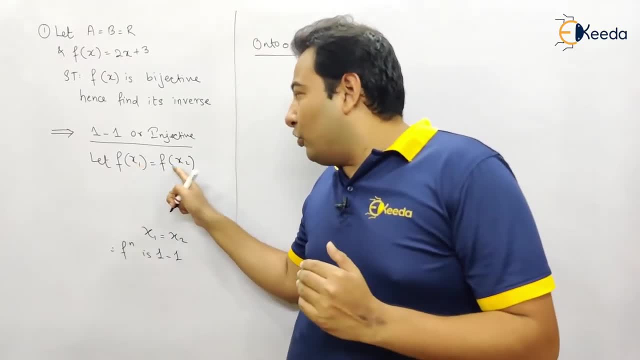 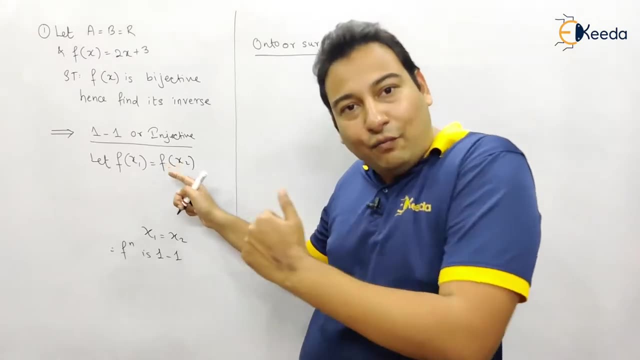 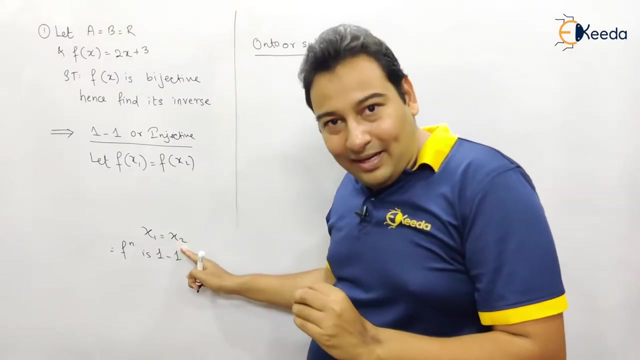 What we are doing. We are starting with there are two different elements with the same image, which is not possible, Because if the elements are different, their image should be different and will conclude that the elements are not different. the elements are same. so that will indicate, if there is only one element- x1, x2- both are same. 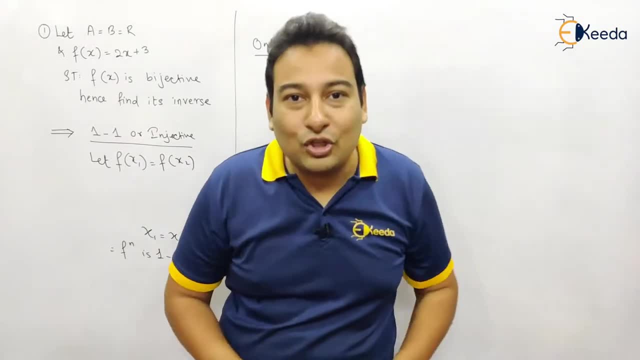 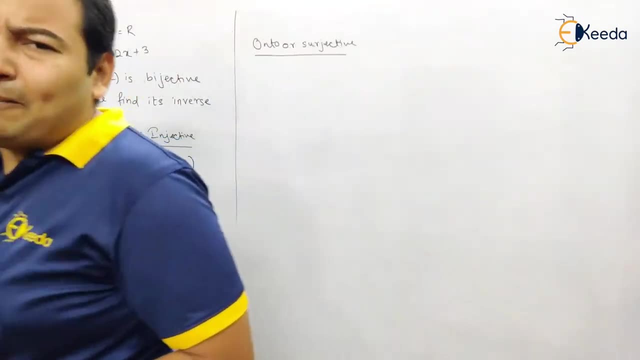 if there is only one element, there is only one image. so this is the procedure. if you understood the logic, what i said, well and good. if not, remember the procedure, we always going to do the same. let us start. so what you're going to do once, we're going to replace this x with x1, so this will 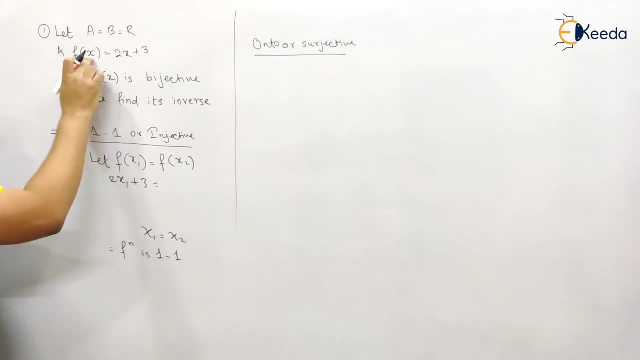 become 2x1 plus 3 and in x we're going to replace x2, so this will become 2x2 plus 3. this will be cancelled. will be left with. 2x1 is equal to 2x2, x1 equal to x2. function is 1 to 1, always step fix. 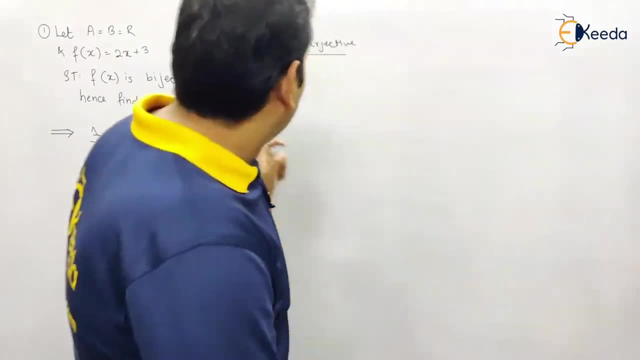 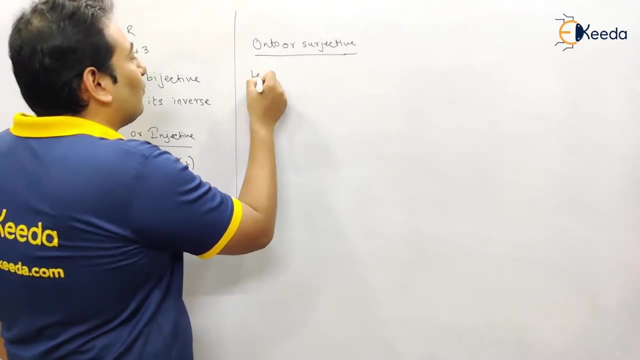 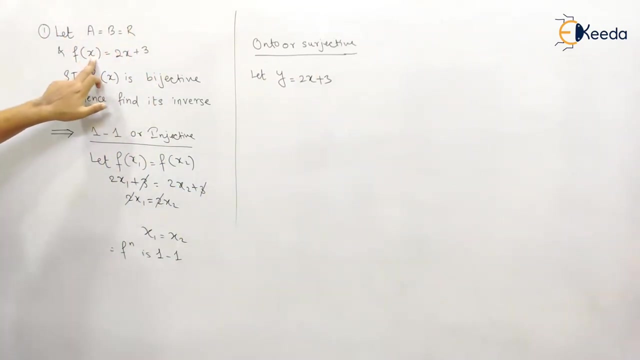 understood the logic. well and good, not remember the procedure. let's move on and let's understand onto, onto or subject to. here we'll always start with let y is equal to 2x plus 3. we'll always start with this because we know f of x is what y, or let's say y is equal to f of x. let's start. 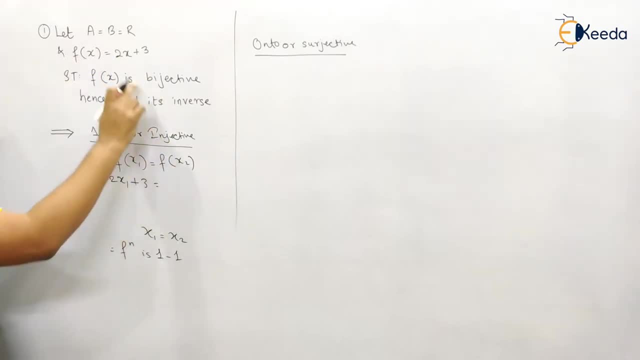 and in x we're going to replace x2, so this will become 2x2 plus 3. this will be cancelled. we'll be left with: 2x1 is equal to 2x2, x1 equal to x2. function is one to one, always step fix. 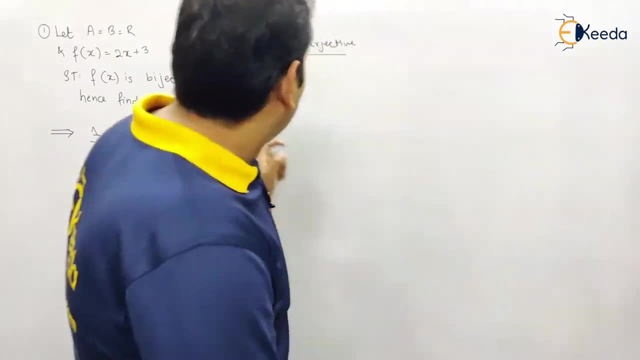 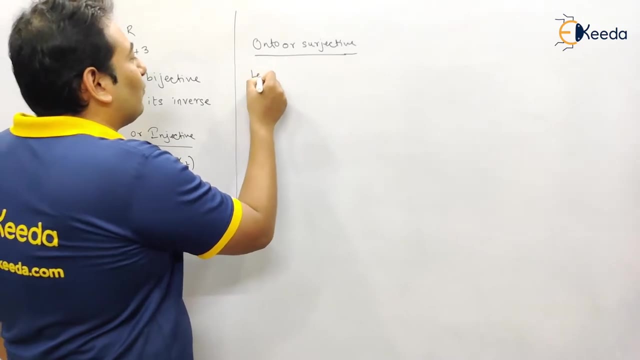 understood the logic. well and good. not remember the procedure. let's move on and let's understand: onto, onto or surject to. here we'll always start with: let y is equal to 2x plus 3. we'll always start with this. why is other people? 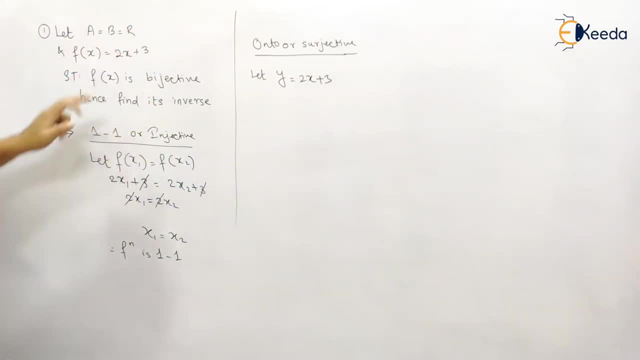 because we know f of x is what why. or let's say: y is equal to f of x. let's start like this: y is equal to f of x. so what is f of x? f of x is 2x plus 3. after doing few steps, what you're going to do, we're going to write it down. 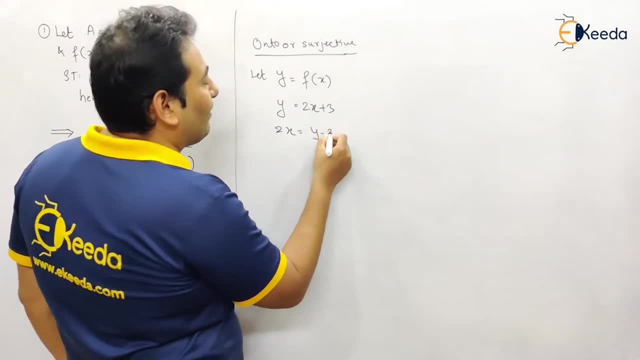 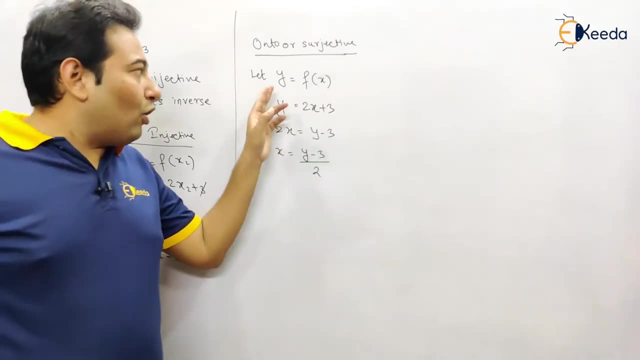 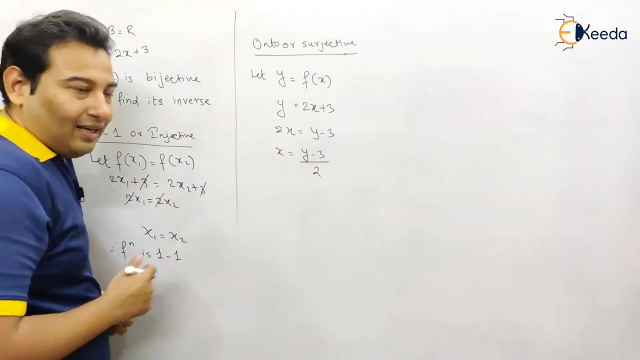 fine, so to x will be y minus 3, so x will be y minus 3 upon 2.. So the procedure is fixed. we'll always start with y equal to and after 4.. some manipulation: we'll write it down as x equal to. now let me write it down a technical statement. 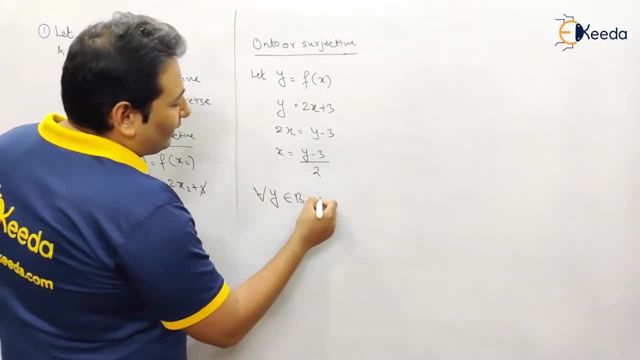 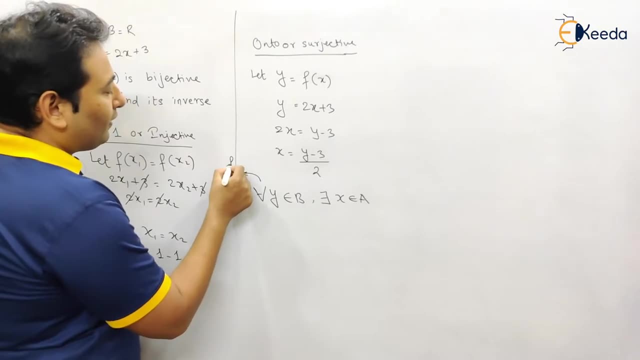 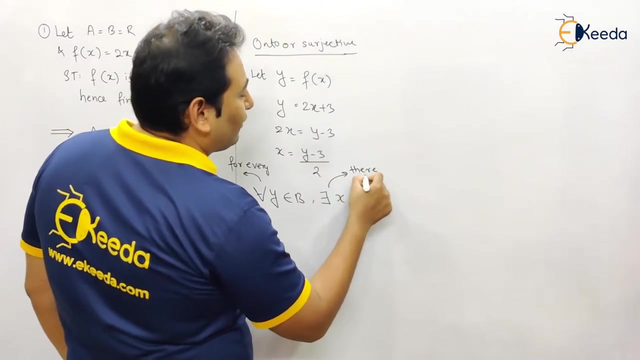 for every y belongs to b, there exists some x belongs to a. this is called for, every this we have seen in the properties of relation, reflex, you and so on. that time, and this is called there exist, and collectively they both are called quantifiers. so remember this: they are called 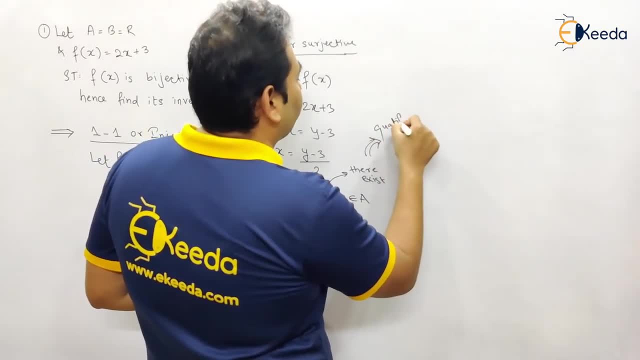 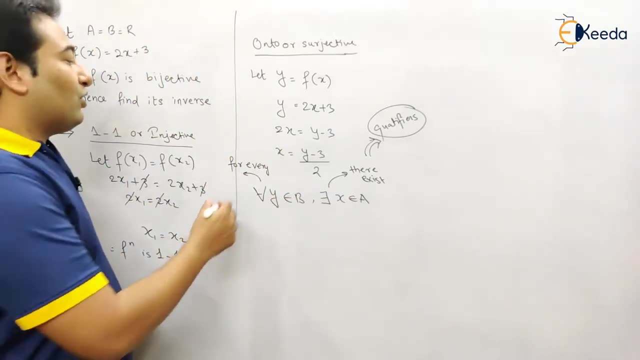 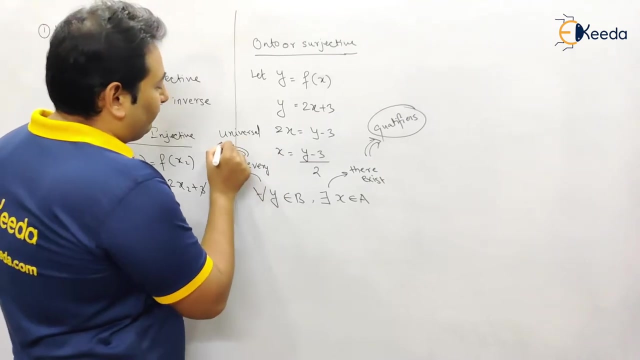 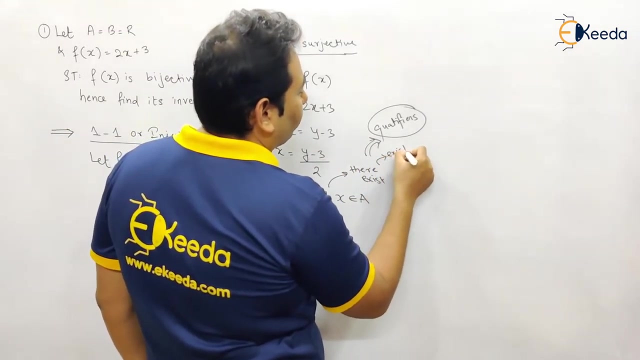 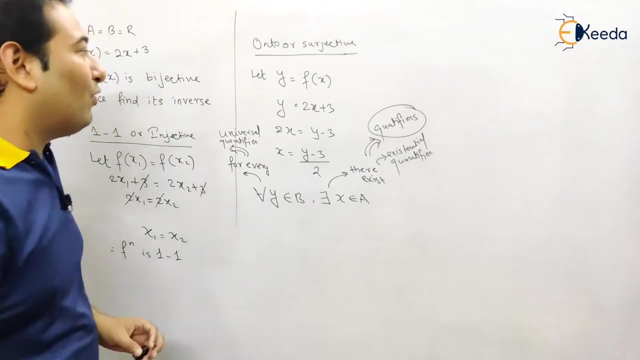 quantifiers. this is your universal quantifier, this is your existential quantifier. so let me write it down: this is your universal quantifier and this is your existential quantifier. now, what is? what do you mean by onto function? onto function says: for every base there should be. 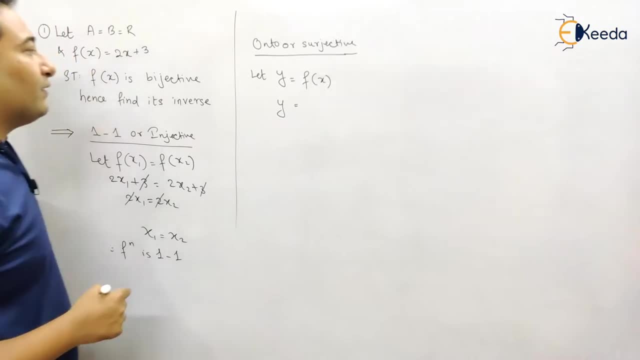 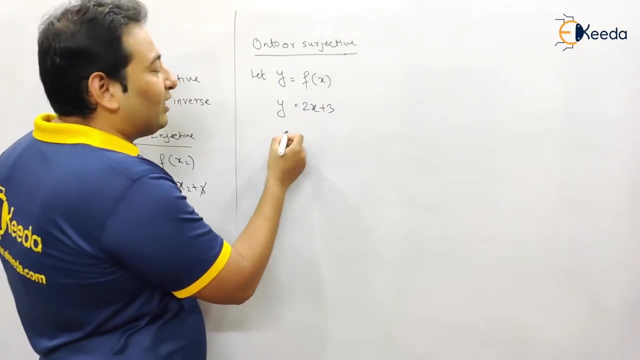 like this: y is equal to f of x. so what is f of x? f of x is 2x plus 3. after doing few steps, what you're going to do, we're going to write it down as x equal to fixed procedure, so 2x will be y minus 3. 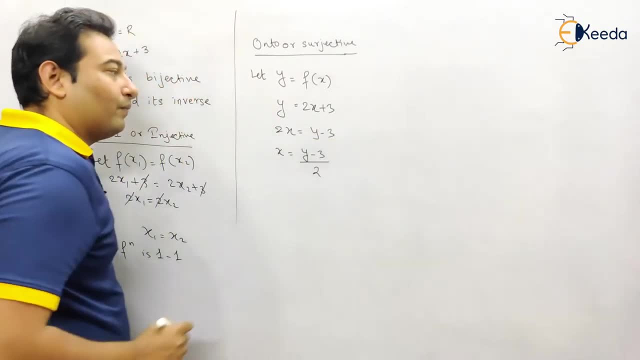 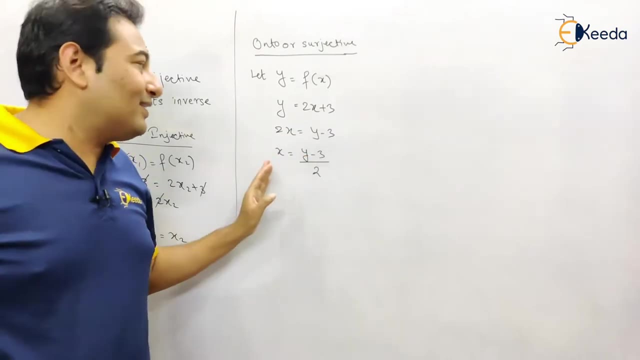 so x will be y minus 3 upon 2, so the procedure is fixed. we'll always start with y equal to and, after some manipulation, we'll write it down as x equal to. now let me write it down a technical statement. for every y is equal to 2x plus 3. we're going to write it down as x equal to 2x plus 3. 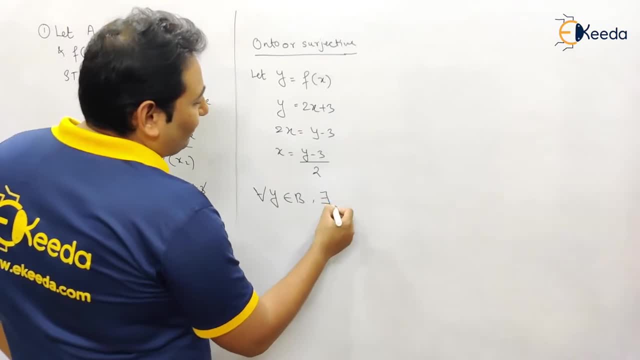 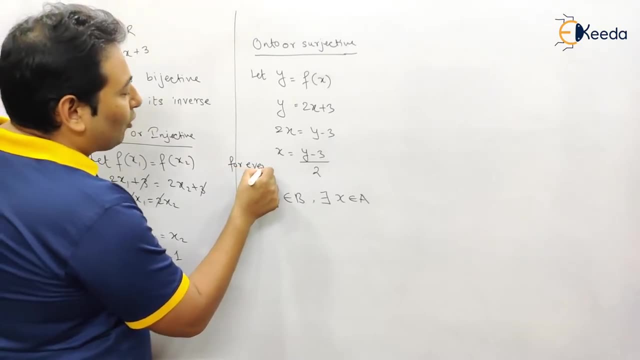 let's see f of x that i times 2 x this way: if r says this, f of x is 2x plus 3, and if x shoe case, try to write this in theㄠ. in this case, if r lost, sometimes f of x is 1. 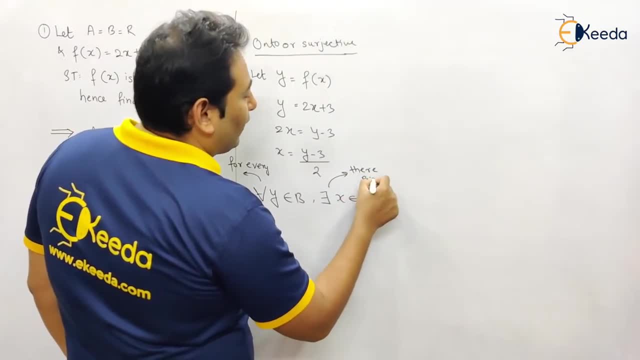 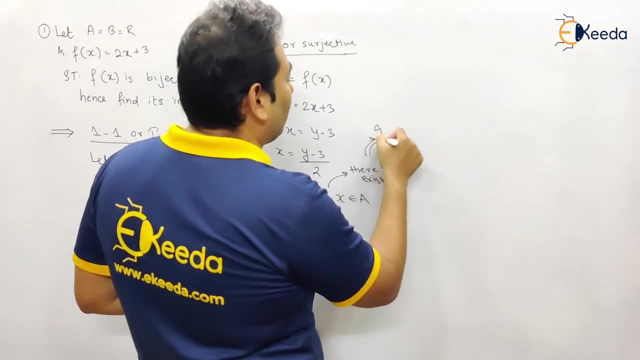 it's 1x. if ser TA, then f. please write this down as 1x times 2x plus 5s plus 6s plus 4s, or if here: if r calls E on all five of them, this x equals to 1s plus 3 plus 4s plus 5s. 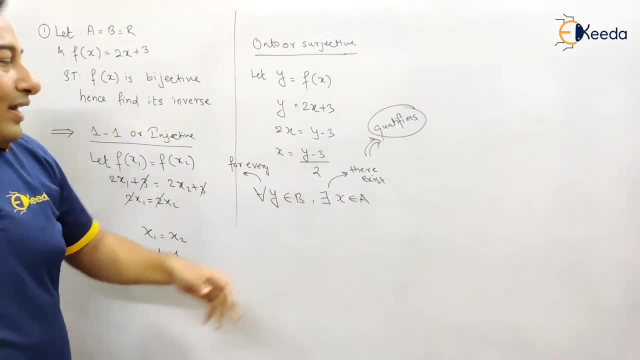 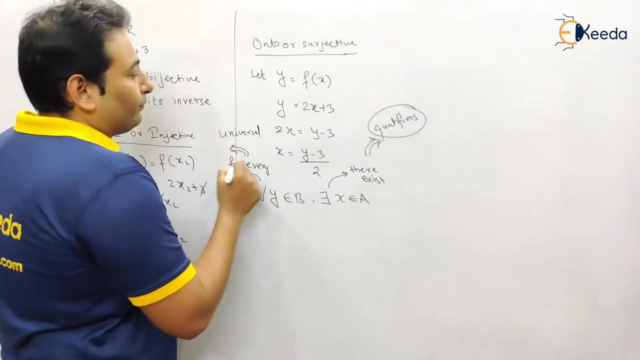 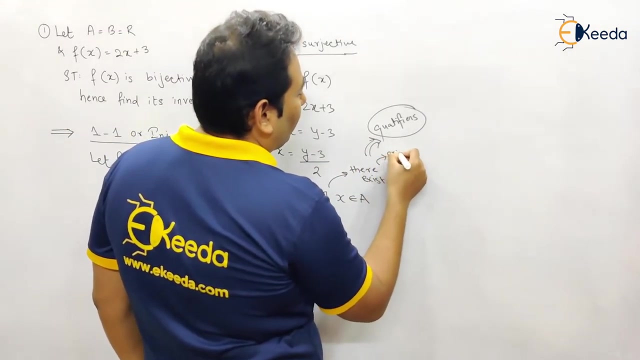 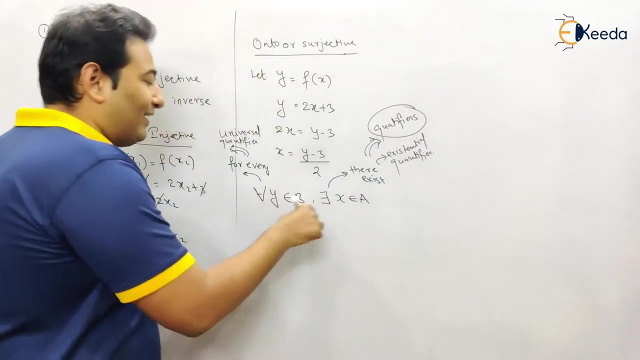 always. This is your universal quantifier, this is your existential quantifier. So let me write it down: This is your universal quantifier and this is your existential quantifier. Now, what do you mean by onto function? Onto function says: for every base, there should be a. 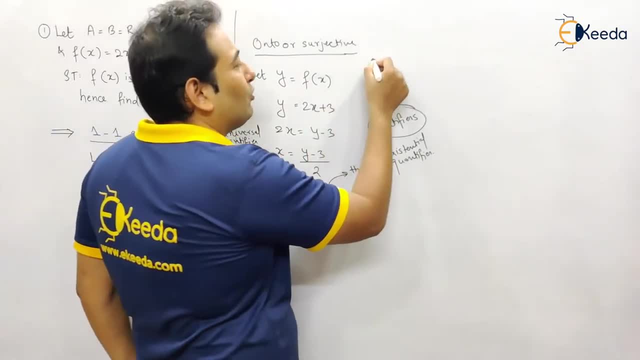 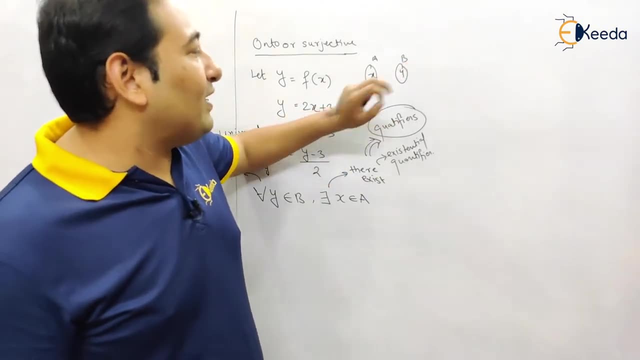 Now, if you put y, see here, suppose here it is a and here it is b. elements of a, we are naming it as x, element of b is y. Now, if you put any value of y, let's say 0,, 1,, 2,, 3,, negative value, any value put, any. 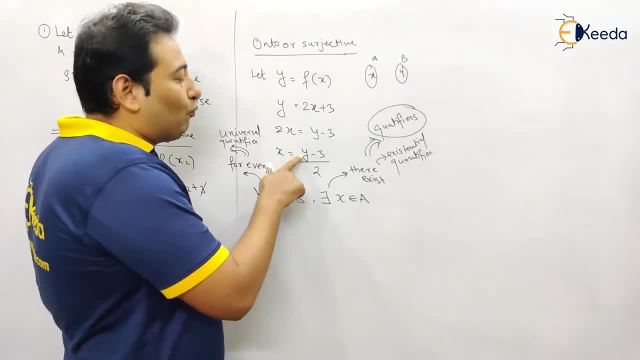 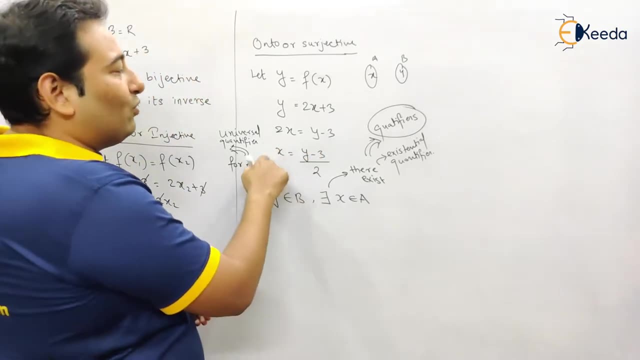 value of y, you will get some value of x. Let's say, if you put y is equal to 1.. So this will become: 1 minus 3 is minus 2, minus 2 upon 2 is minus 1.. So if you put y is equal to 1, you will get x equal to 1.. 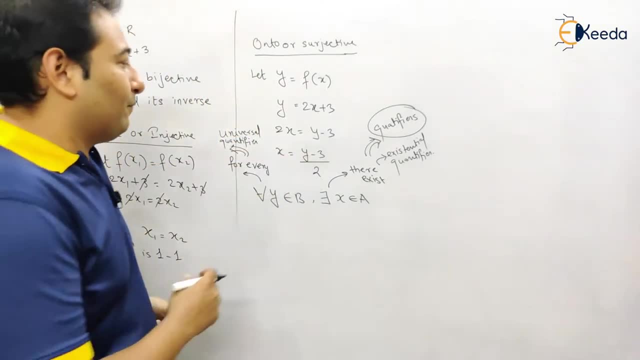 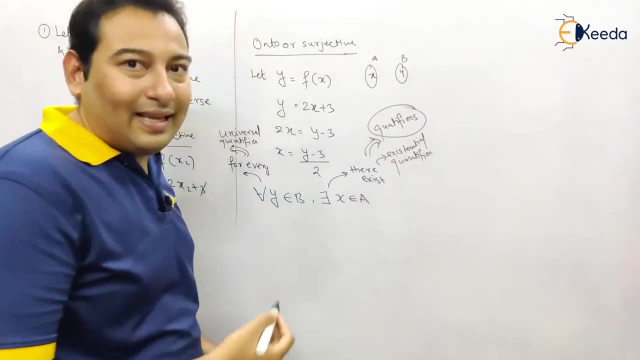 a. now if you put y, if see here, suppose here it is a and here it is b. elements of a, we are naming it as x. element of b is y. now if you put any value of y, let's say 0, 1, 2, 3- negative value. 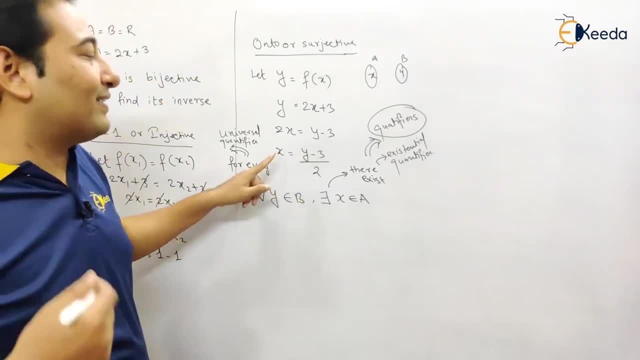 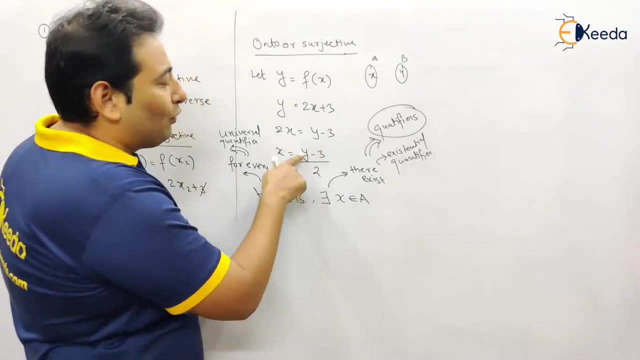 any value. put any value of y, you will get some value of x. let's say: if you put y is equal to 1, you'll become 1 minus 3 is minus 2. minus 2 upon 2 is minus 1. so if you put y is equal to 1, you'll. 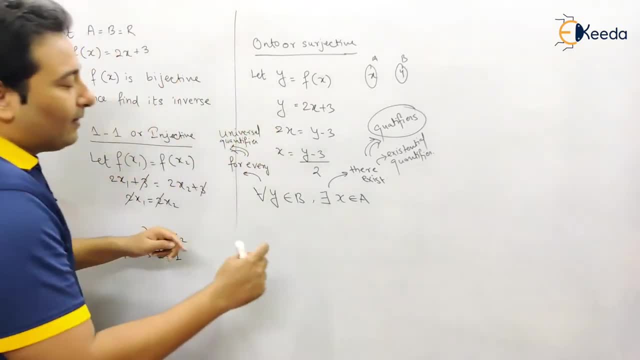 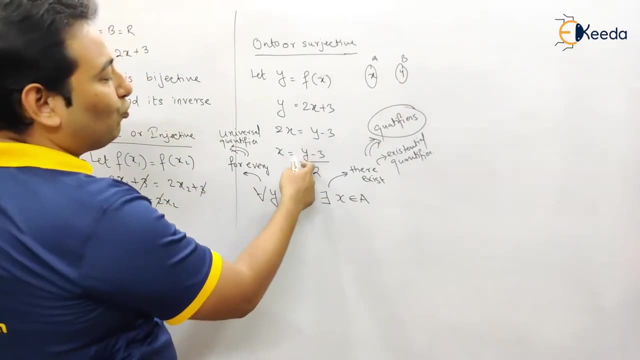 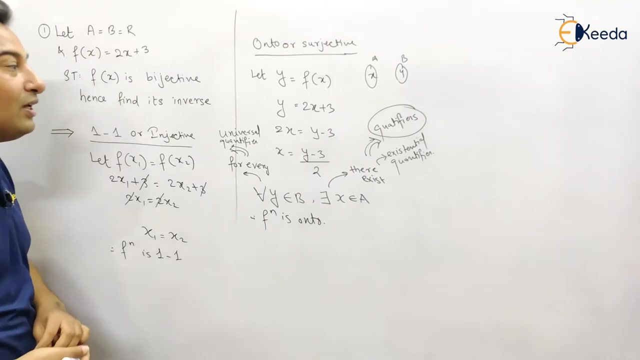 get x equal to 1. so this is the statement, the means. for every y belongs to b. for every y belongs to b, there exists some x belongs to a. you put any y, you'll get some x. therefore, the function is onto. is this clear? so what is the procedure? we'll start with y equal to. we'll write it on as x. 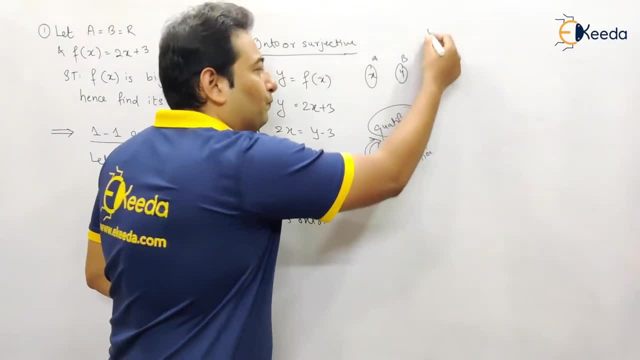 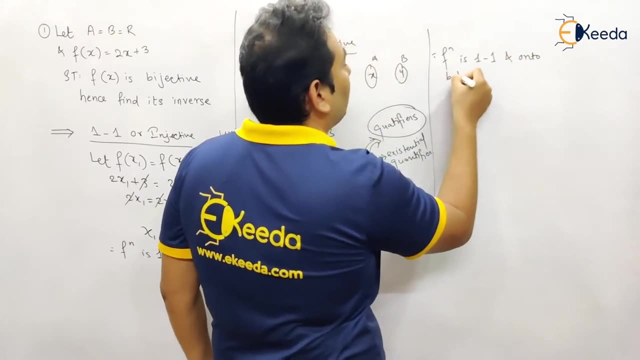 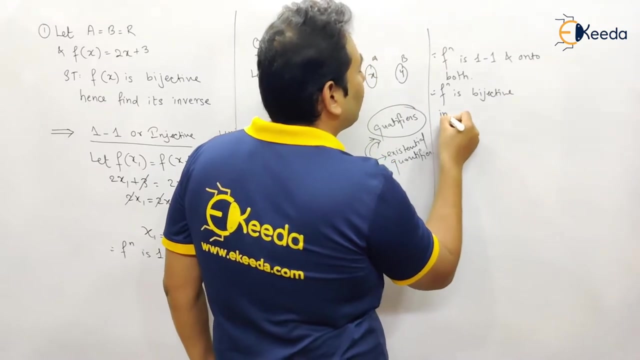 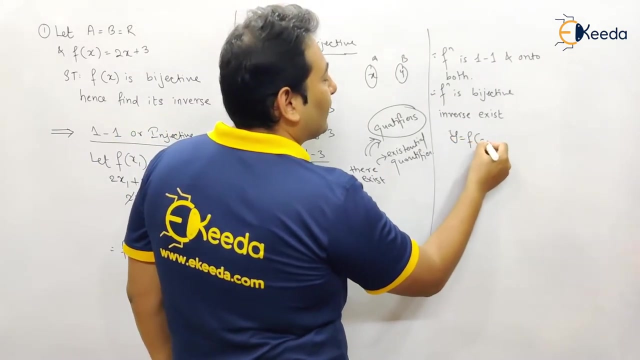 equal to and after that, this is statement. then the function is onto, since the function is one to one, and onto both. therefore, function is bijective. and since the function is bijective, inverse exist. and what is the inverse? you'll start with the same statement. y is equal to f of x. so what is x, f inverse, y for inverse? again, you're going to start with. 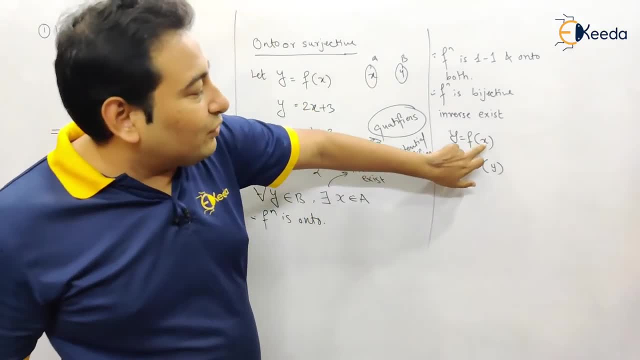 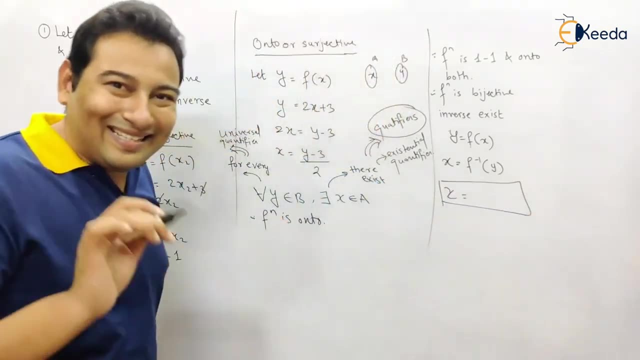 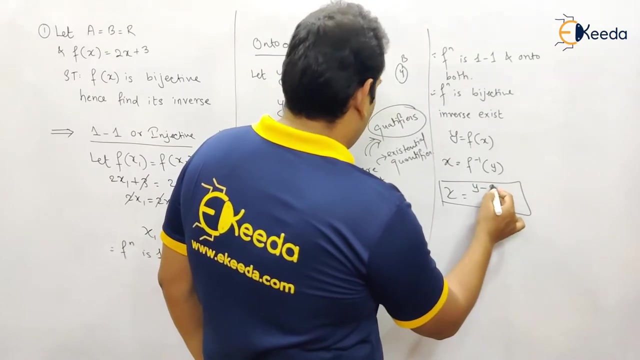 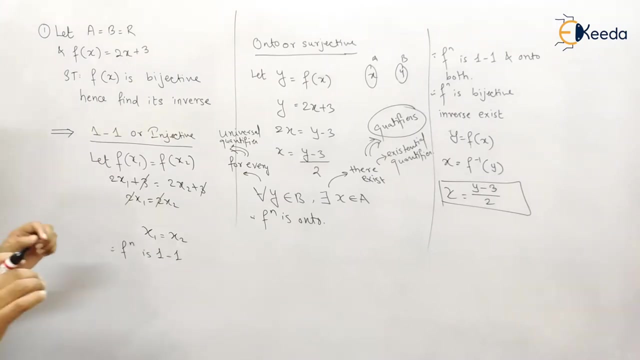 the same statement. y is equal to f of x. x will be 1 minus 3, x is equal to 1 minus 3, x is equal to this. F will go to that side, will become F inverse Y and simply, simply, without thinking, simply just write it on as it is. that is your inverse story over, that's it. whatever is the answer that you. 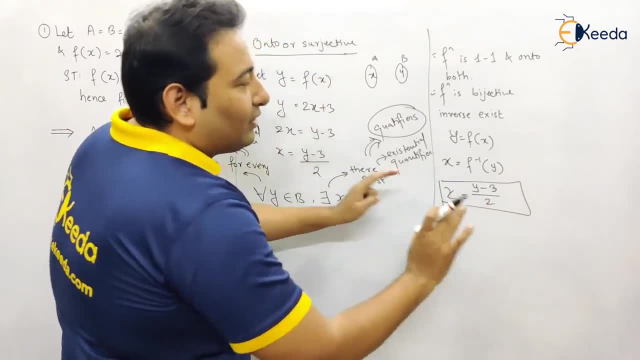 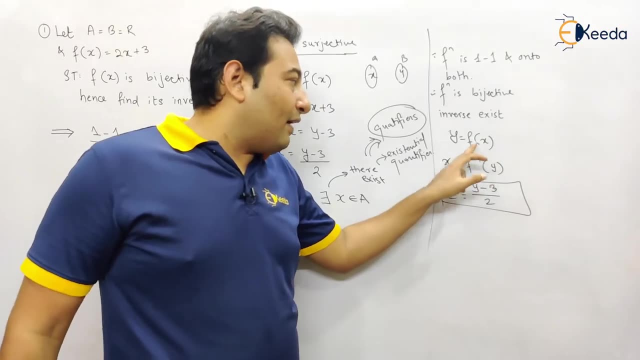 getting here. just simply write it on as it is and the story over. that is your inverse. so what is the procedure? of? inverse Y is equal to F of X, F will be X will be F. inverse Y, and simply write it on this and the story is over. this is your inverse. so that is it done with the problem. hope you. 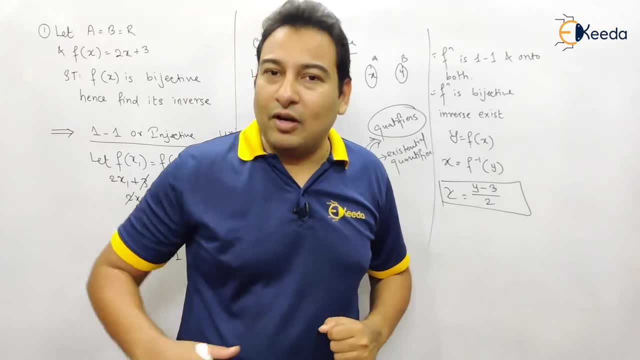 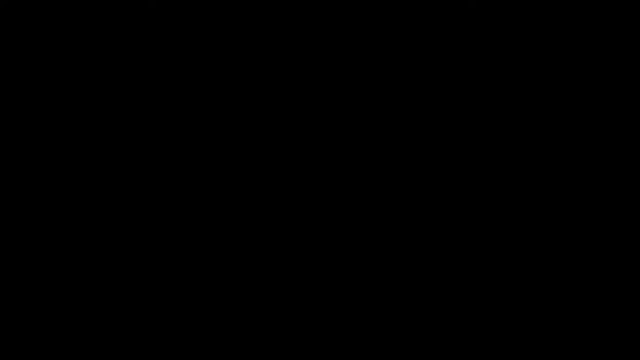 understood. in the next video we'll see one more example of the same type. thank you you.